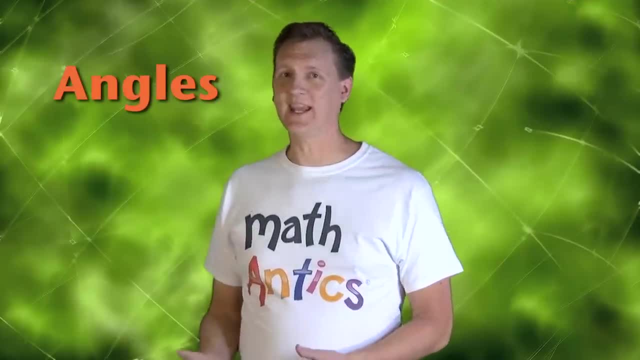 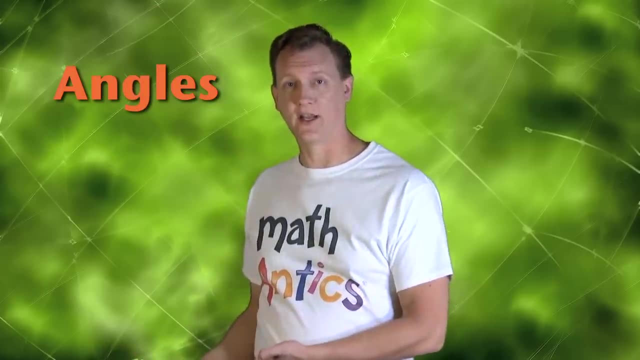 something like that. right, But when it comes to angles, we can't use a ruler to measure them or use units like centimeters. And that's because angles aren't about length. Angles are about rotation, And to measure how much something is rotated we use a special unit. 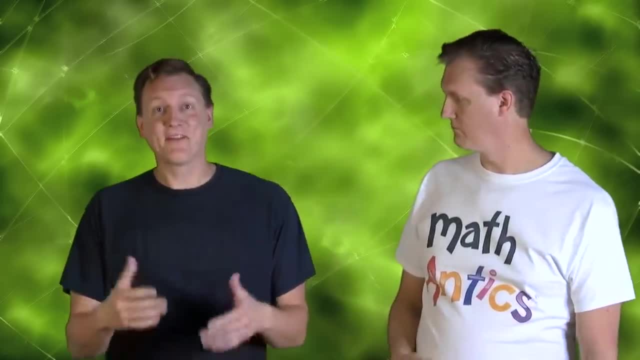 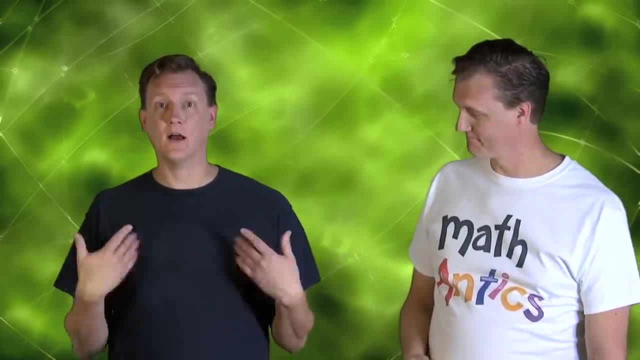 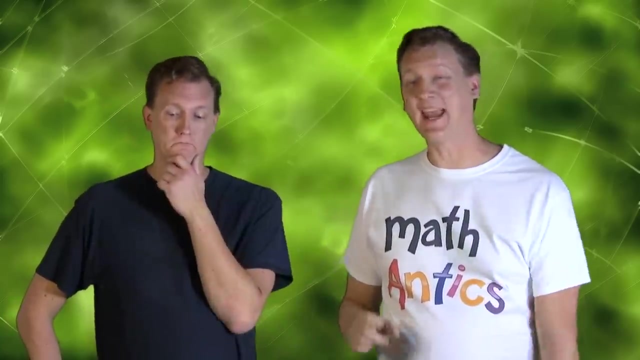 called degrees. Now hold on a second. I thought degrees were used to measure how hot or cold something is, You know, like it's a hundred degrees outside today. Ah, now, that is a good point, you smart looking fella. The word degree is used for a lot of different things, so it can be a. 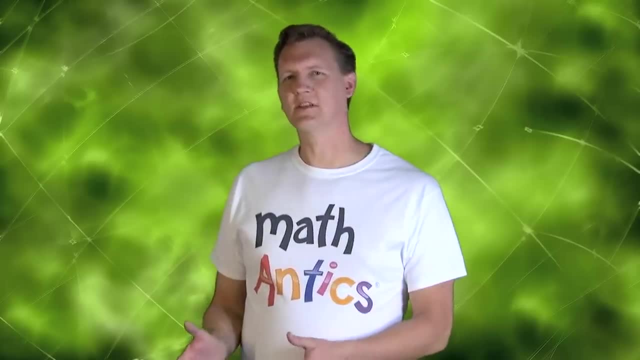 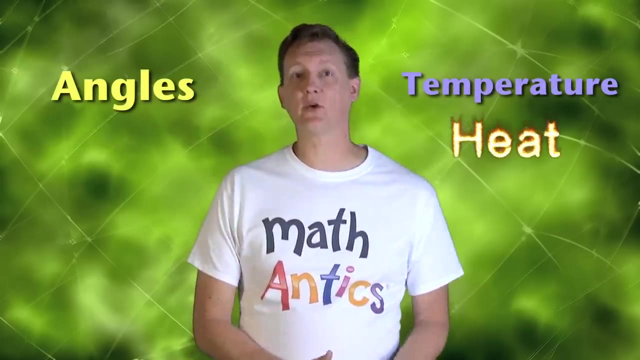 little confusing. sometimes It makes more sense if you just think of a degree as a small amount of something. For temperature, a degree is a small amount of heat, But for angles a degree is a small amount of rotation And there's a special math symbol for degrees. 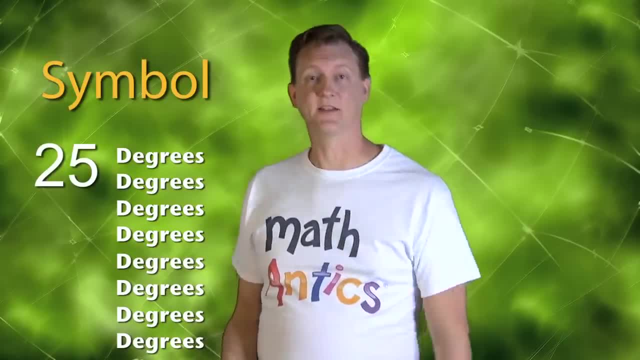 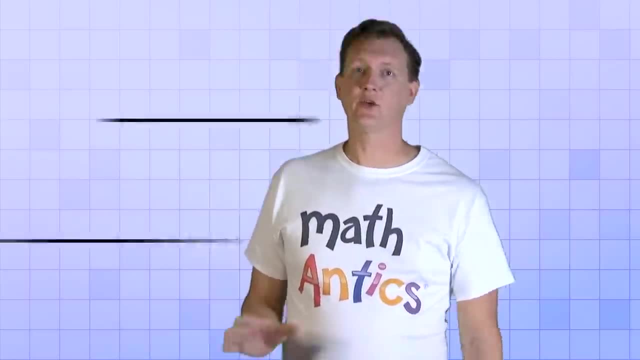 that we use instead of writing the word degrees over and over again. It's this little circle that you put after the number and up near the top To see how we use degrees to measure angles. let's get two rays that point in exactly the same direction. Then let's put one ray directly on top of the other one so it looks. 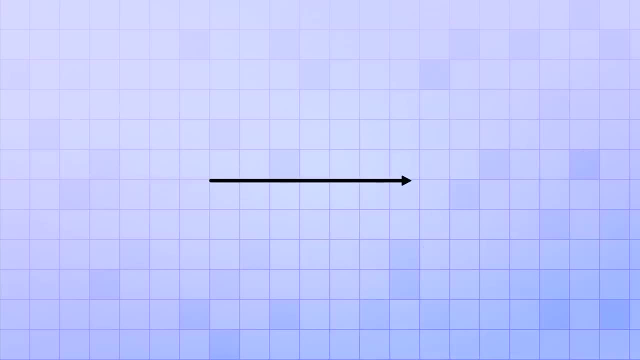 like there's only one ray there, even though there's really two. Now let's take the ray on top and rotate it just a tiny amount counter-clockwise. This point on the ray will be our axis or center of rotation. It's just like the point at the center of a clock that stays stationary while the hands 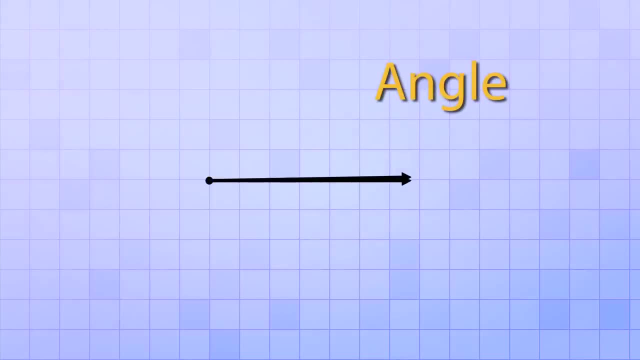 rotate around it, Our rays now form an angle that measures 1 degree And, as you can see, 1 degree is a really small angle. We need to zoom in on it to see that it really is an angle. In fact, you might wonder if there could be any angles smaller than 1 degree. 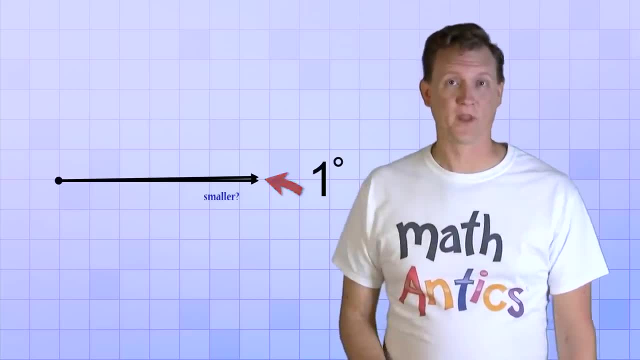 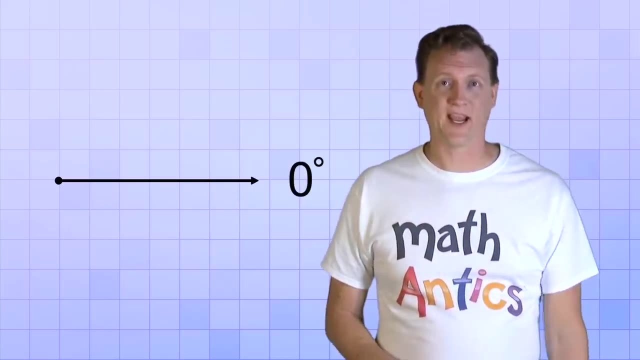 Yup, there sure are, And we saw one just a second ago, Before we rotated our top ray, when our rays were exactly on top of each other. that was a zero degree angle, And there's a whole range of tiny fraction angles in between zero. 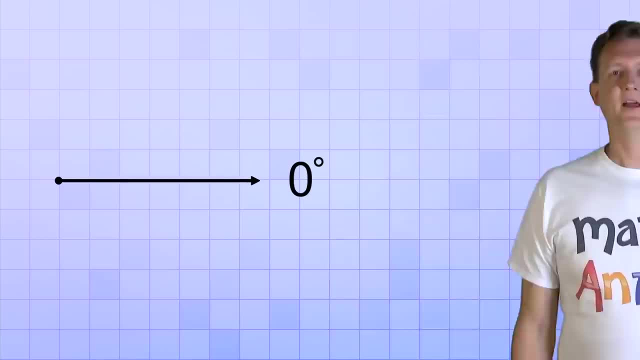 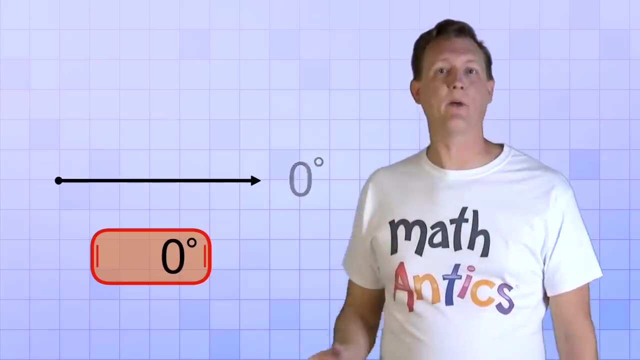 and 1 degree, But we aren't going to learn about them in this video. Instead, we're going to keep on rotating our top ray and watch the angle get bigger and bigger. This special readout here will tell us how many degrees our angle measures. 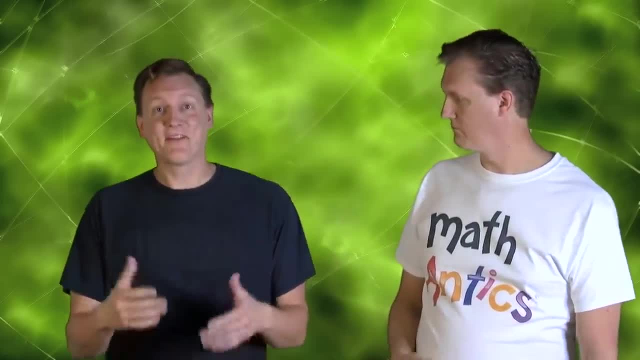 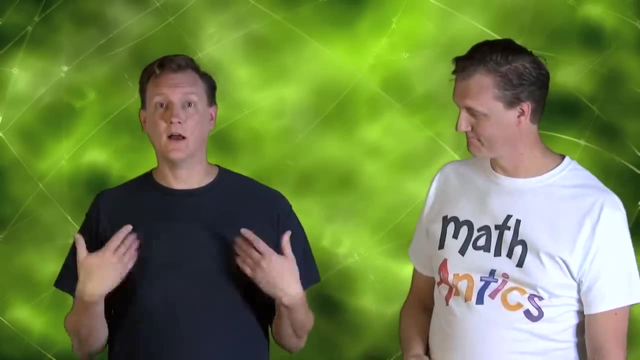 called degrees. Now hold on a second. I thought degrees were used to measure how hot or cold something is. You know, like it's a hundred degrees outside today. Ah, now, that is a good point, you smart looking fella. The word degree is used for a lot of. 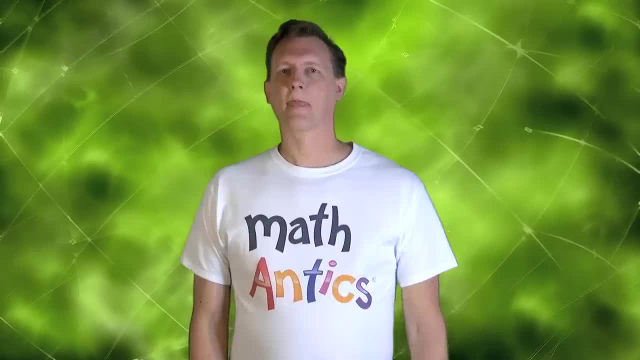 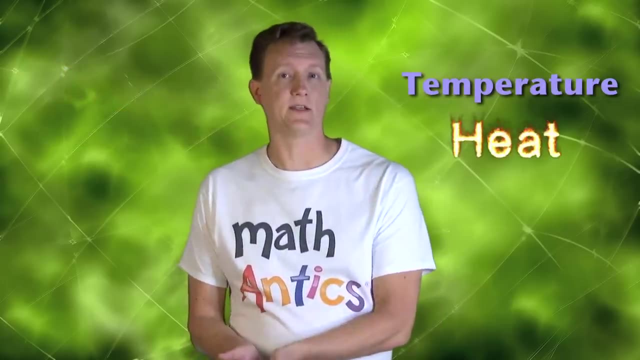 different things, so it can be a little confusing. sometimes It makes more sense if you just think of a degree as a small amount of something. For temperature a degree is a small amount of heat, But for angles a degree is a small. 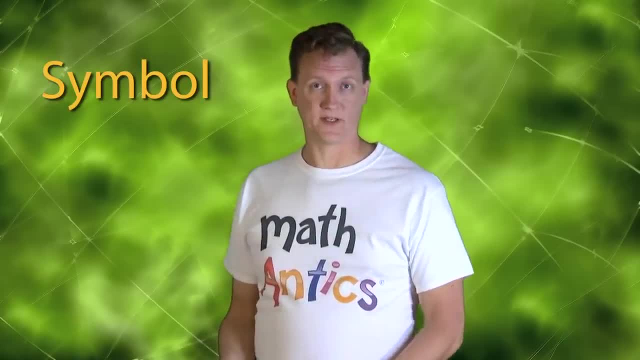 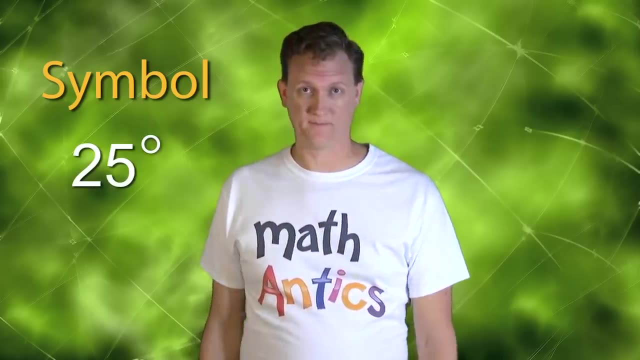 amount of rotation. And there's a special math symbol for degrees that we use instead of writing the word degrees over and over again. It's this little circle you put after the number and up near the top To see how we use degrees to measure angles. let's get two rays that point in exactly. 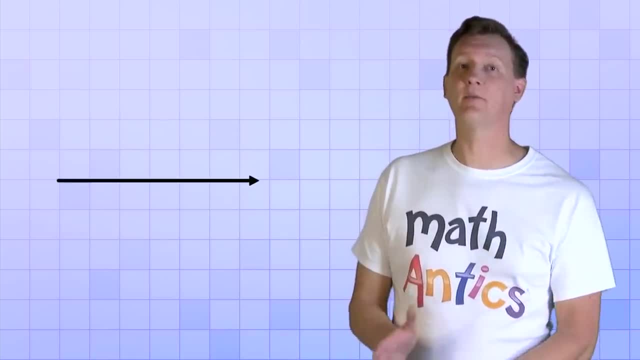 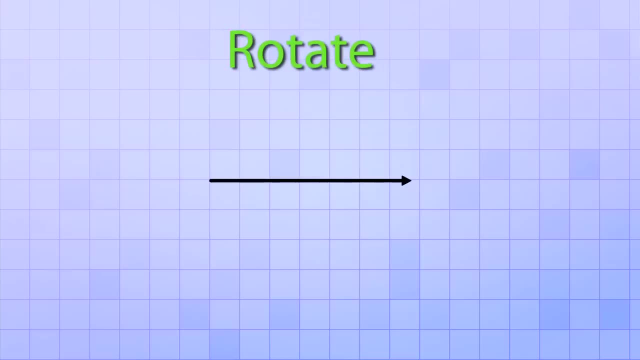 the same direction. Then let's put one ray directly on top of the other one, so it looks like there are only one ray there. Now let's take the ray on the top and rotate it just a tiny amount, counterclockwise. This 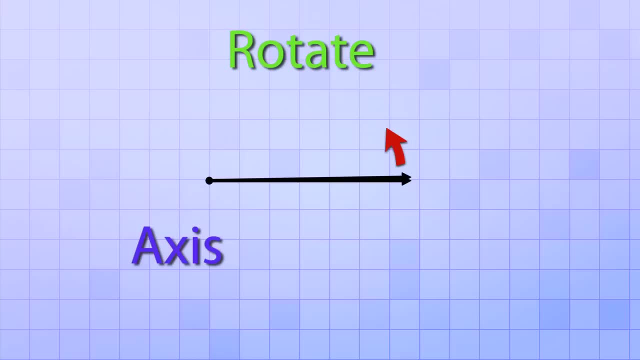 point on the ray will be our axis or center of rotation. It's just like the point at the center of a clock that stays stationary while the hand stays on its desk. That's adalah ع никогда rotate around it. Our rays now form an angle that measures one degree And, as you can see, 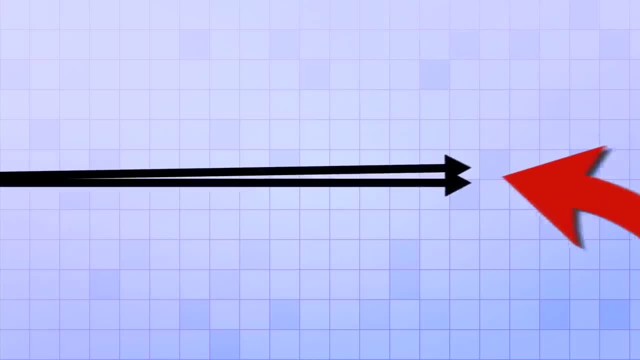 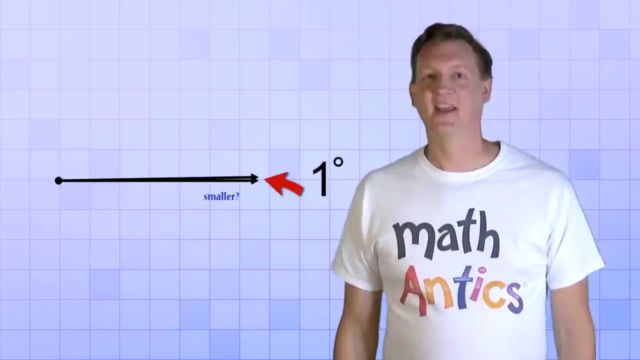 one degree is a really small angle. We need to zoom in on it to see that it really is an angle. In fact, you might wonder if there could be any angles smaller than one degree. Yup, there sure are, And we saw one just a second ago, Before we rotated our top ray. 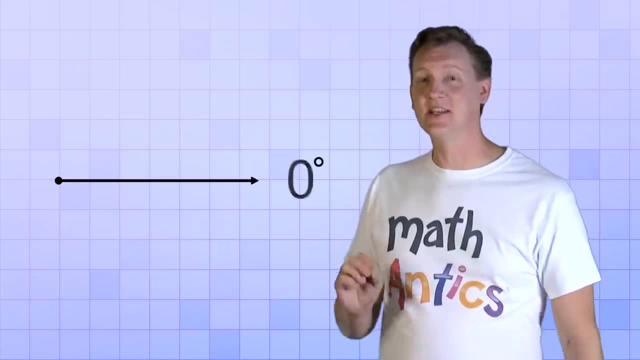 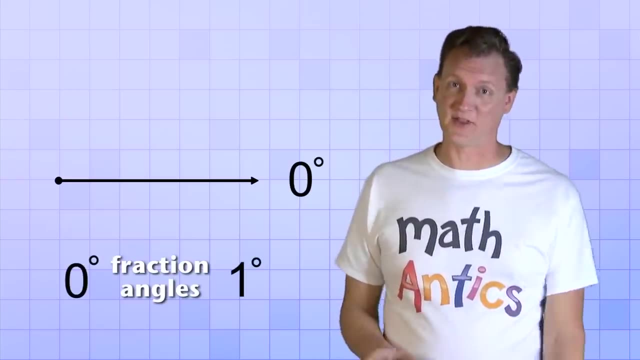 when our rays were exactly on top of each other. that was a zero degree angle, And there's a whole range of tiny fraction angles in between zero and one degree, But we aren't going to learn about them in this video. Instead, we're going to keep on rotating our top ray and watch the angle get. 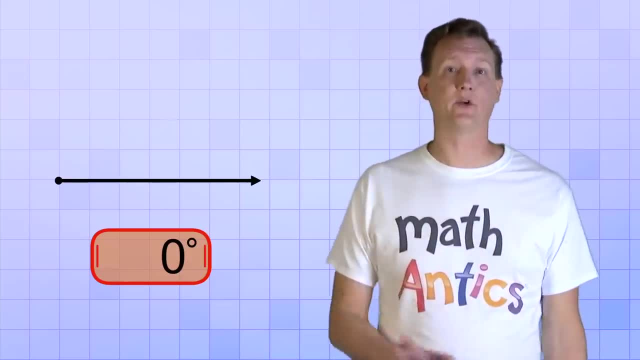 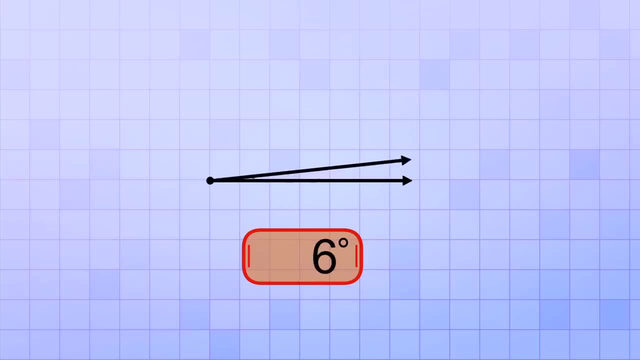 bigger and bigger. This special readout here will tell us how many degrees our angle measures. Now let's start out slow: One degree: two, three, four, five, six, seven, eight, nine and ten. Now let's hold it there for a second. So this is what ten degrees looks like. 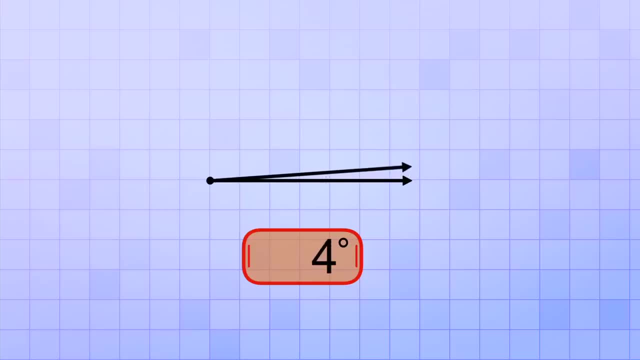 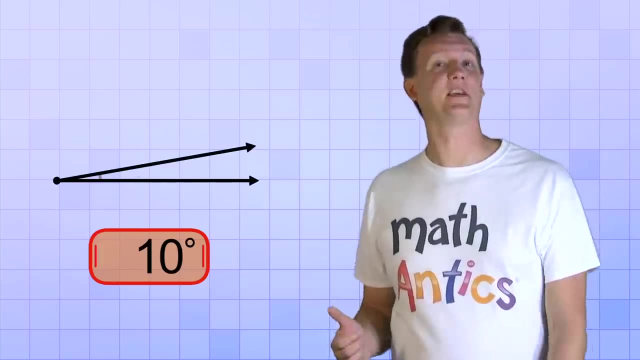 Now let's start out slow. 1 degree: 2,, 3,, 4,, 5,, 6,, 7,, 8,, 9, and 10.. Now let's hold it there for a second. So this is what 10 degrees looks like. 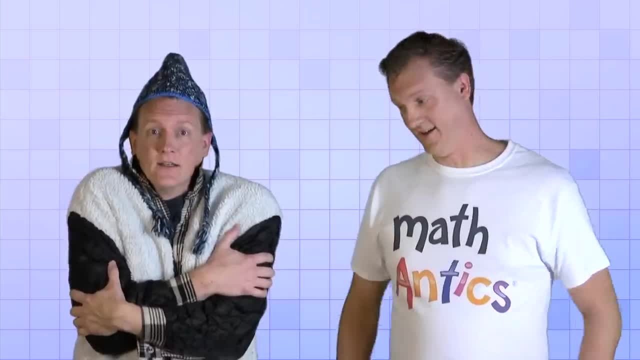 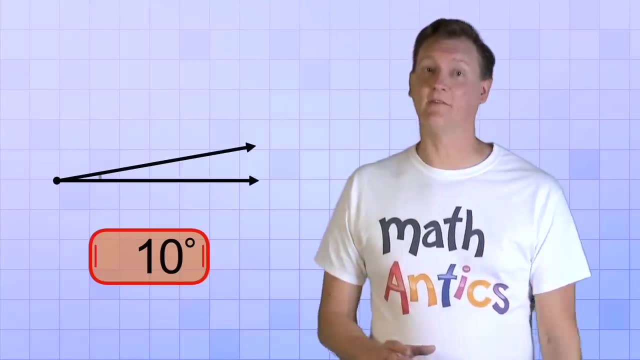 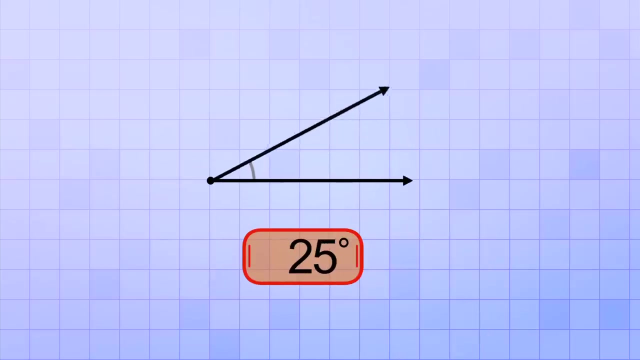 10 degrees, That's f-f-freezing. Huh, Guess, you're not as smart as I thought after all. So we can see that a 10 degree angle is still a very small angle. So let's keep going, but a little bit faster this time. Alright, that's 15 degrees, 20,, 25,, 30,, 35,, 40, and 45.. Now 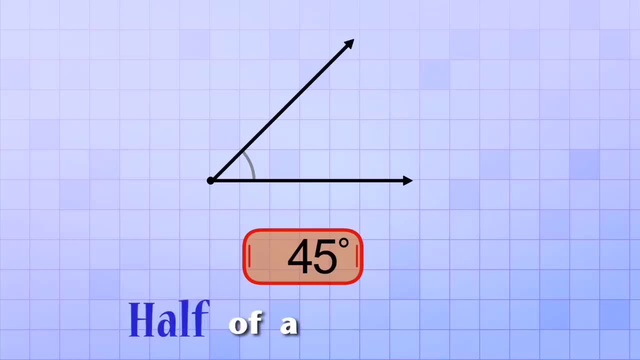 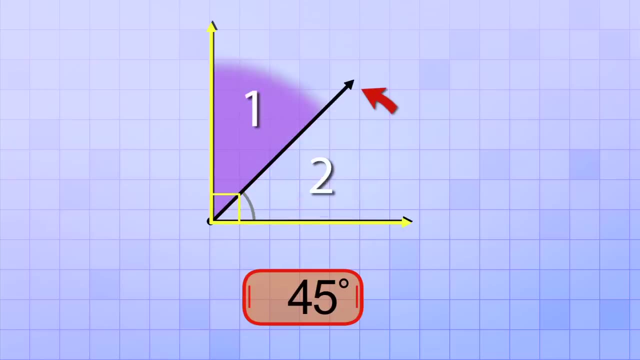 45 degrees is a special angle because it's exactly half of a right angle. If we draw a right angle in the same spot, you can see that our ray cuts it into two equal parts. So if 45 degrees is half of a right angle, can you guess how many degrees a right angle? 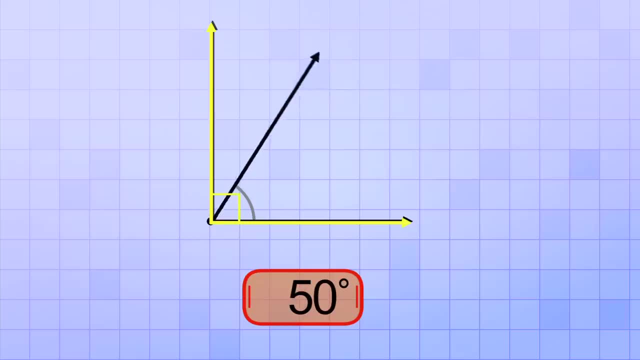 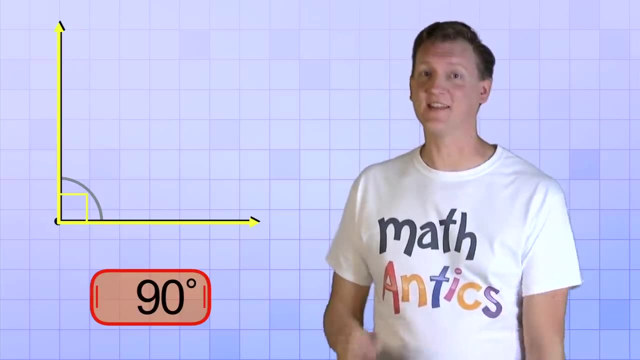 is. Let's keep on rotating to see if you're right: 50,, 60,, 70,, 80, and 90.. Yep, a right angle is exactly 90 degrees And that is super important to memorize because right angles 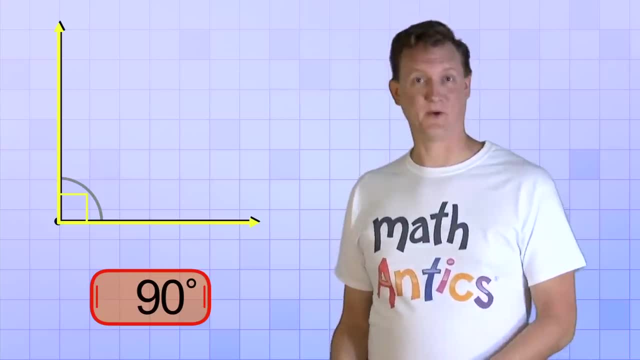 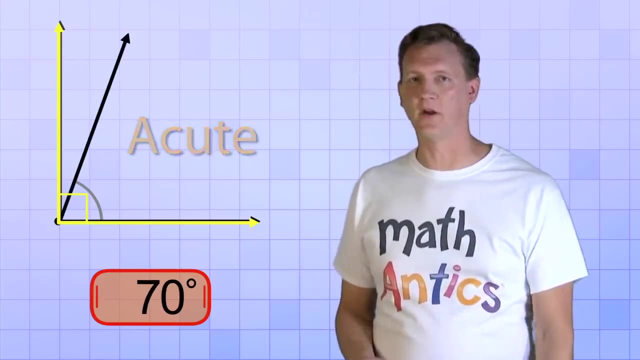 are used all the time in geometry. Okay, so do you remember from our last video that all angles less than a right angle are called acute angles? So this means that all the angles that we've seen so far that are between 0 and 90 degrees are called acute angles, All angles below everything we've seen、. 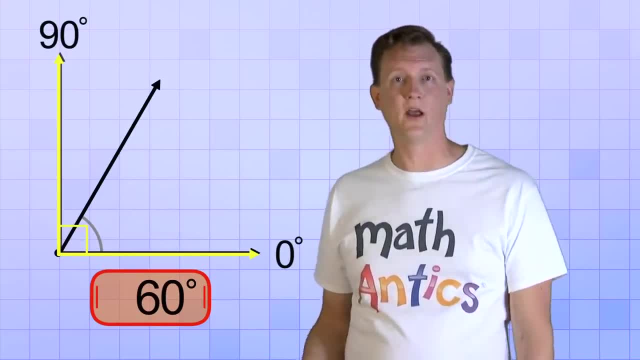 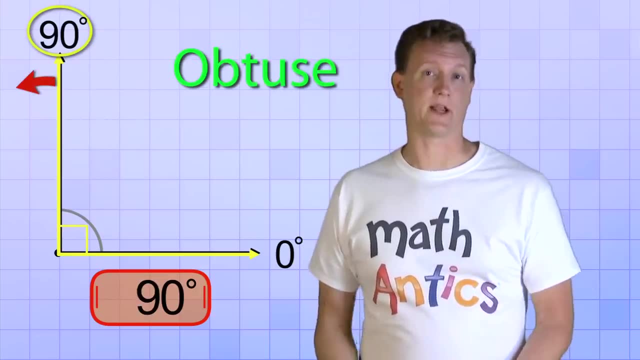 degrees, like 10,, 30,, 45,, 60 and so on, are acute angles, But if we keep on rotating our ray past 90 degrees, we'll start forming obtuse angles because they're greater than a right angle. Ready, Here we go…. 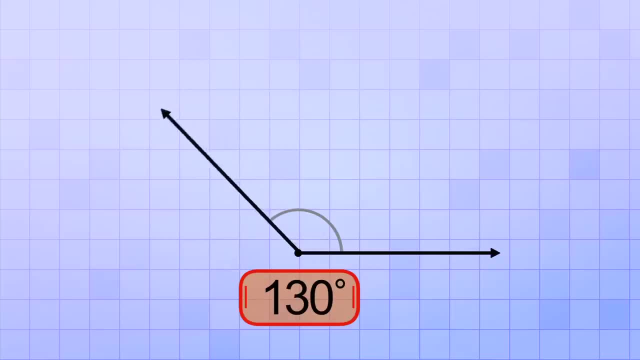 100 degrees, 110,, 120,, 130,, 140,, 150,, 160,, 170 and 180.. Aha, Does this look familiar? Yup, it's a straight angle, like we learned about in the last video. 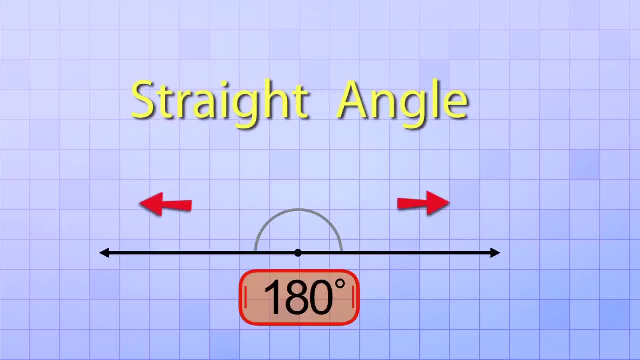 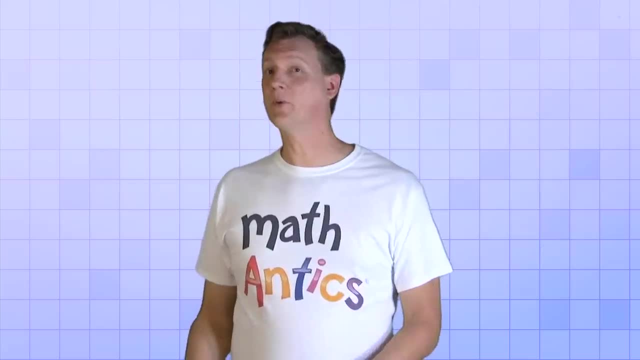 The rays point in exactly opposite directions and the angle they form is 180 degrees, and that's also a really important angle measurement to memorize. Now, before we go on, let's quickly review the important angles and regions that we've looked at so far. 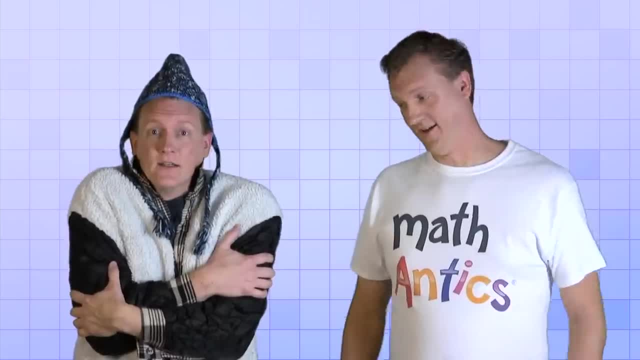 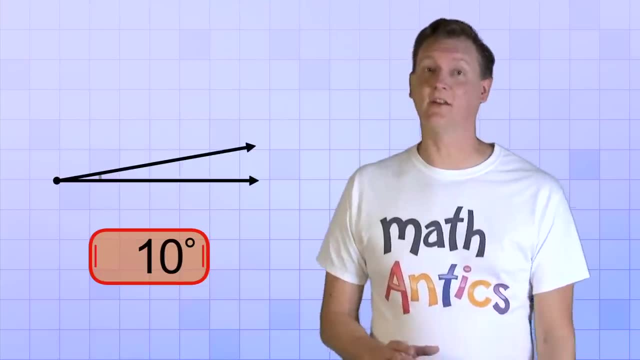 Ten degrees, That's f-f-freezing. Huh, Guess, you're not as smart as I thought after all. So we can see that a ten degree angle is still a very small angle. So let's keep going, but a little bit faster this time. Alright, that's fifteen degrees. 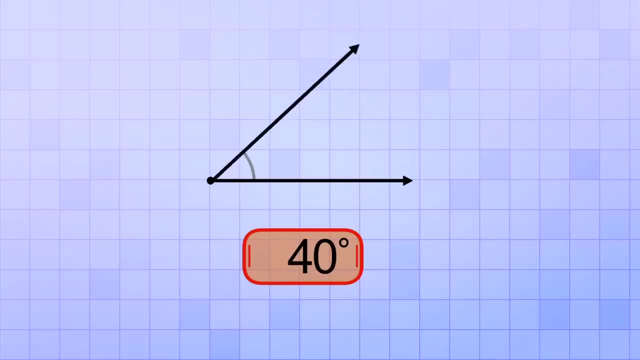 twenty, twenty-five, thirty, thirty-five, forty and forty-five. Now, forty-five degrees is a special angle because it's exactly half of a right angle. If we draw a right angle in the same spot, you can see that our ray cuts it into two equal parts. 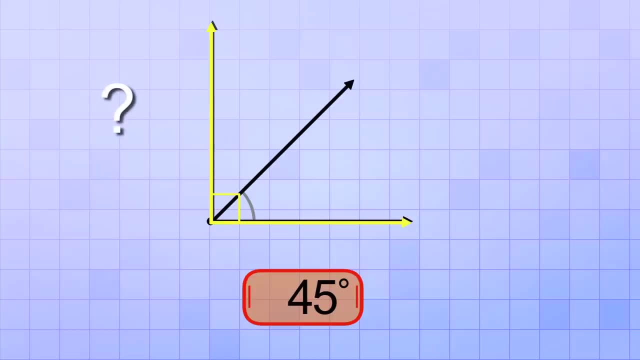 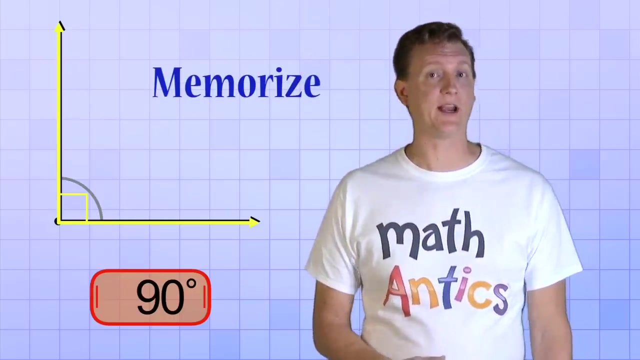 So if forty-five degrees is half of a right angle, can you guess how many degrees a right angle is? Let's keep on rotating to see if you're right. Fifty, sixty, seventy, eighty and ninety: Yup, a right angle is exactly ninety degrees, And that is super important to memorize, because right. 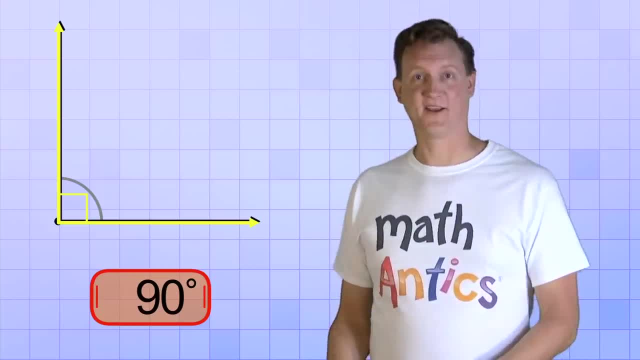 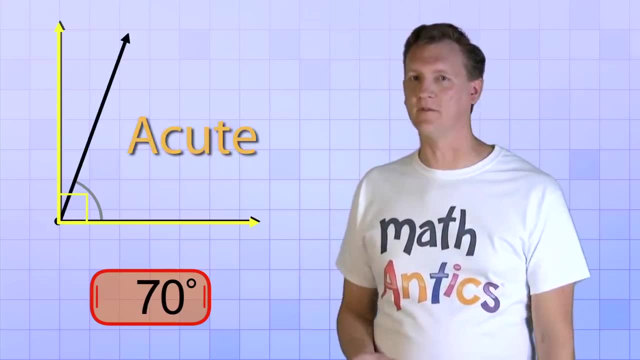 angles are used all the time in geometry. Okay, do you remember from our last video that all angles less than a right angle are called acute angles? So that means that all the angles we've seen so far that are between zero and ninety degrees, like ten, thirty, forty-five. 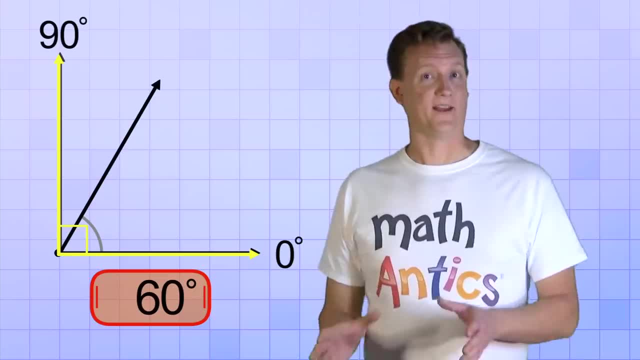 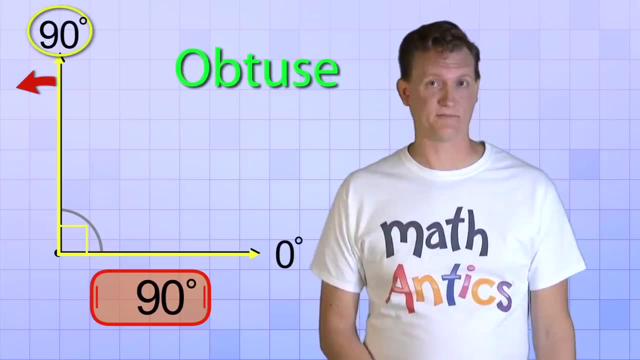 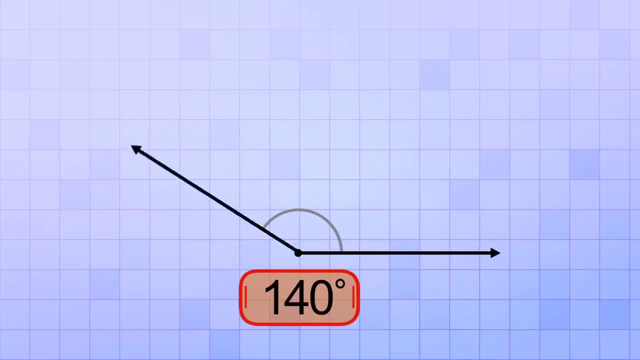 sixty and so on are acute angles, But if we keep on rotating our ray past ninety degrees, we'll start forming obtuse angles, because they're greater than a right angle. Ready, Here we go. One hundred degrees, one ten one, twenty one, thirty one, forty one, fifty one, sixty one, seventy. 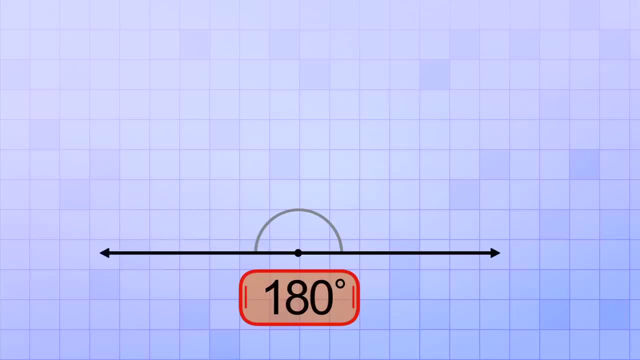 and one eighty. Aha, Does this look familiar? Yup, it's a straight angle. like we learned about in the last video, The rays point in exactly opposite directions and the angle they form is a hundred and eighty degrees, And that's also a really important angle measurement to memorize. 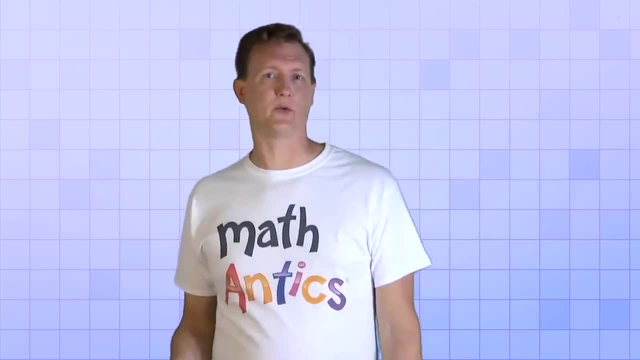 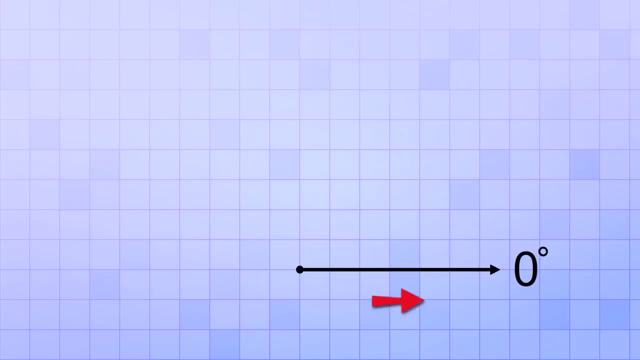 Now, before we go on, let's quickly review the important angles and regions that we've looked at so far. Our angle measurement is zero degrees when the rays point in exactly the same direction. It's ninety degrees when the rays are perpendicular and form a right angle, And it's a hundred and eighty degrees when they 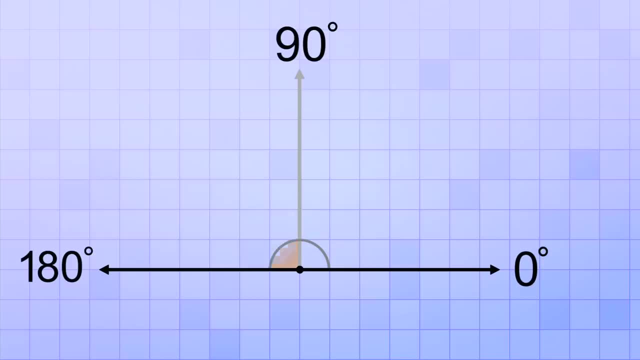 point in opposite directions and form a straight angle. In this region between ninety and one eighty we find obtuse angles, And in this region between zero and ninety we find acute angles. One important acute angle is forty-five degrees, since it's half of a right angle. 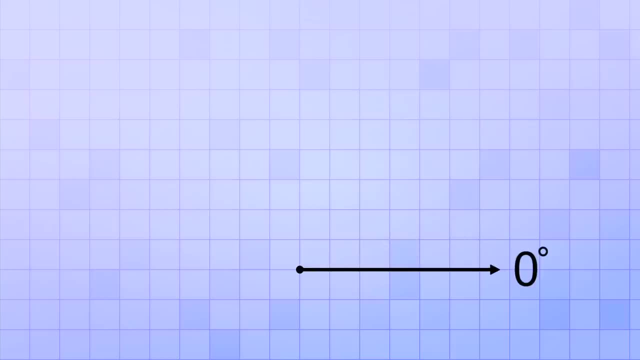 Our angle measurement is 0 degrees when the rays point in exactly the same direction, It's 90 degrees when they're perpendicular and form a right angle. And it's 180 degrees when they're perpendicular and form a right angle. And it's 180 degrees when they point in opposite directions and form a straight angle. 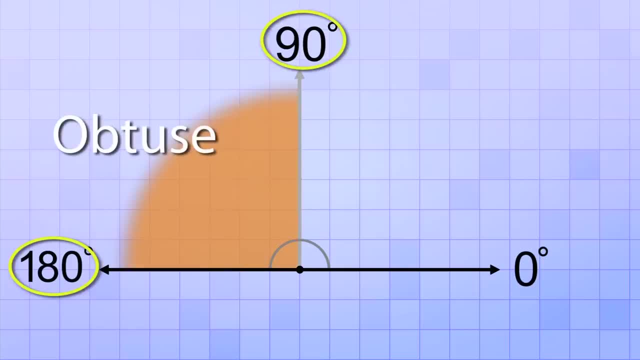 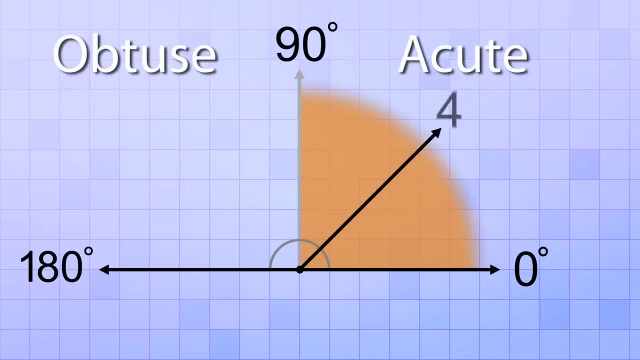 In this region between 90 and 180, we find obtuse angles, And in this region between 0 and 90, we find acute angles. One important acute angle is 45 degrees, since it's half of a right angle. 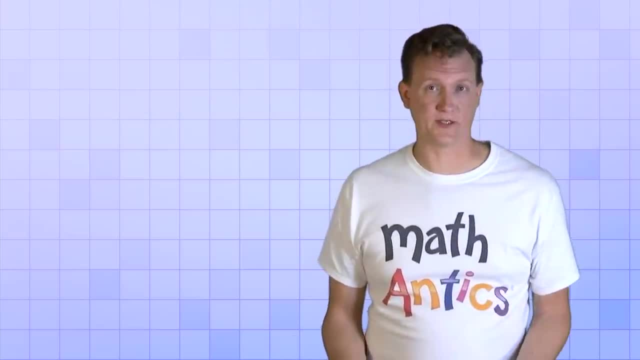 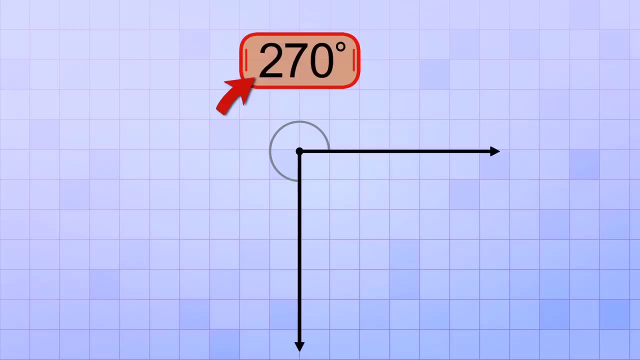 Alright, then let's continue rotating past 180 degrees. Our angle readout keeps getting higher, and the next important angle we come to is this one: 270 degrees. It also forms a right angle, but it points down instead of up. Let's keep going, because another really important angle is just around the corner. 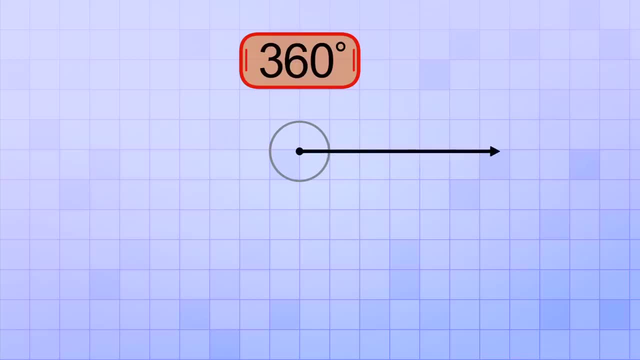 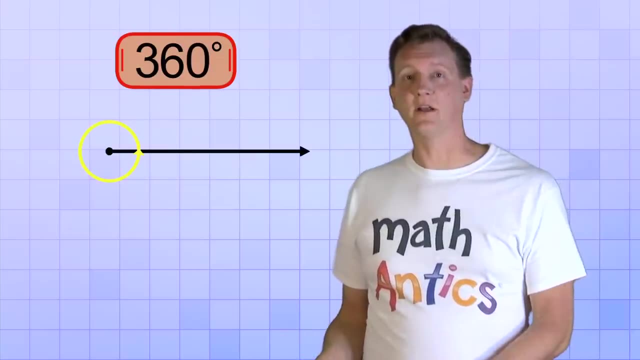 and it's coming up right about now. We rotated our ray all the way around the axis and now it's back to where we started. Now you might be wondering: if we're back to where we started, then why is our counter reading 360 degrees instead of 0 degrees like before? 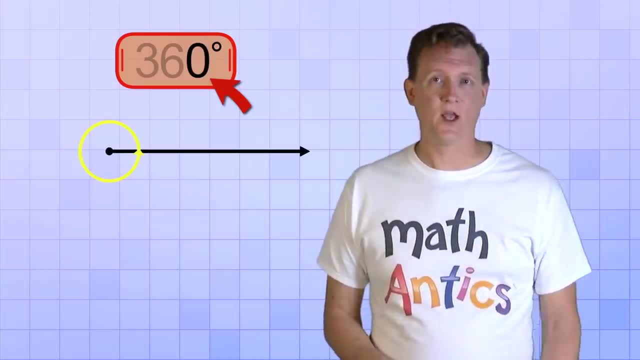 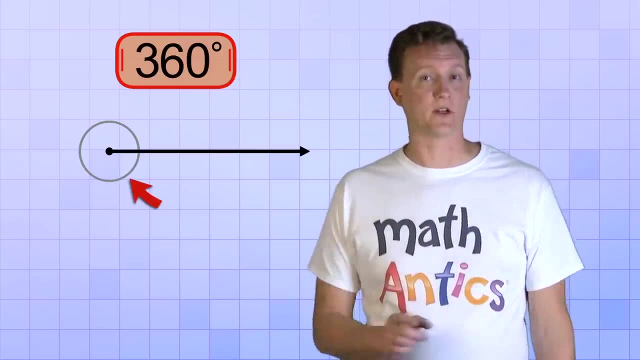 And the answer is that, even though our rays are back to the same place, we had to rotate our top ray 360 degrees to get there, And you can see that our angle arc now forms a complete circle. So 360 degrees is the angle that represents a full circle. 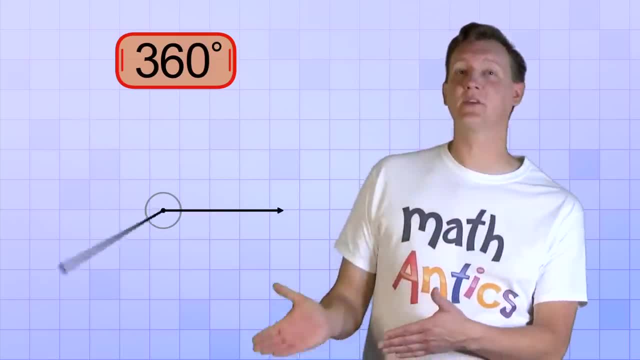 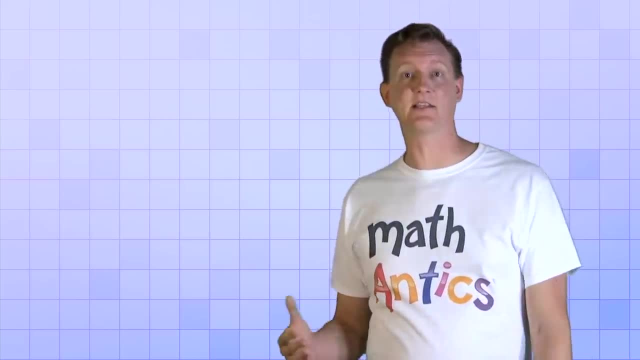 Rotating 360 degrees brings you all the way around the circle to the point that you started from. Okay, now that you know what degrees are and you've seen how they relate to the size of an angle, we need to learn how to actually measure an angle without this fancy readout that we have here. 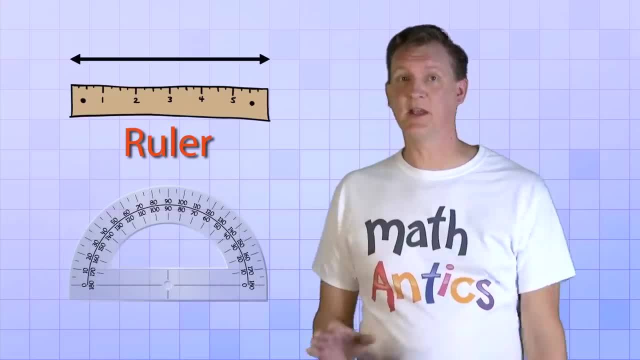 Just like a ruler can be used to measure the length of a line, a special tool called a ruler can be used to measure the length of a line. a special tool called a ruler and a special tool called a protractor can be used to measure angles. 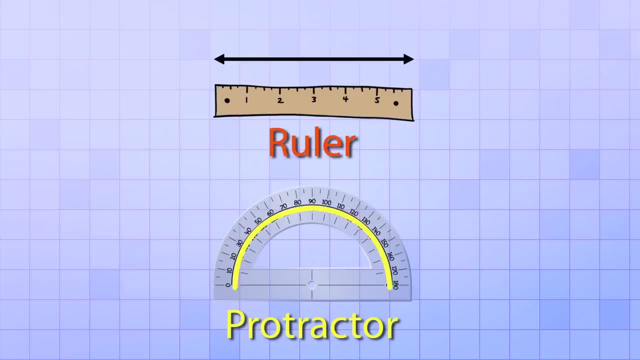 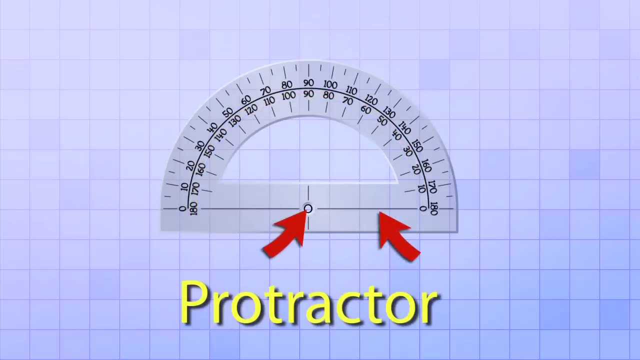 A protractor is similar to a ruler, but it's curved into a half circle so that it can measure rotation around an axis point. A protractor also has a straight edge with a hole or a dot in the middle that represents the axis or center of rotation. 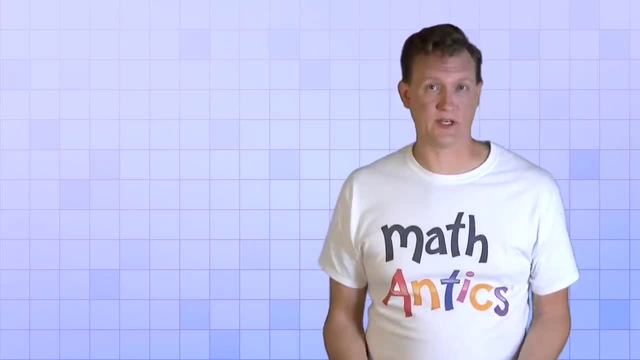 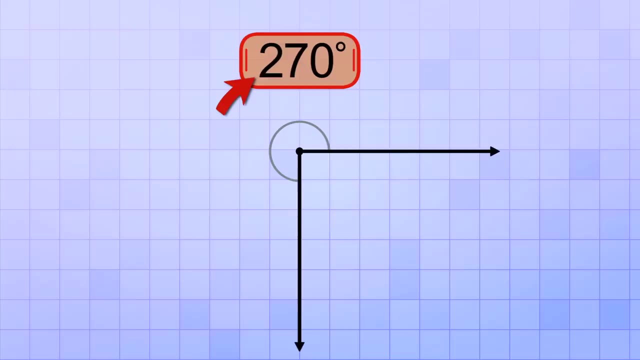 Alright, then let's continue rotating past one hundred and eighty degrees, Our angle readout keeps getting higher, and the next important angle we come to is this one: Two hundred and seventy degrees. It also forms a right angle, but it points down instead of up. 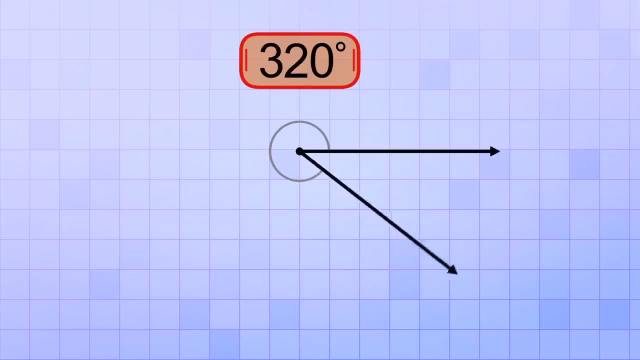 Let's keep going, because another really important angle is just around the corner And it's coming up right about now. We rotated our ray all the way around the axis and now it's back to where we started. Now you might be wondering if we're back to where we started. 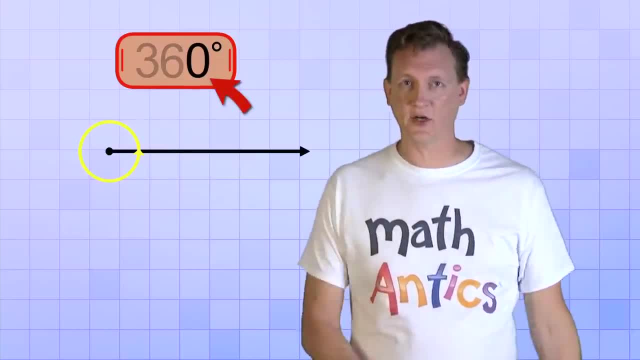 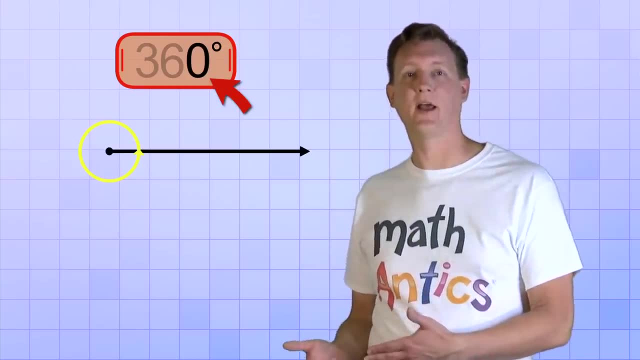 then why is our counter reading three hundred and sixty degrees instead of zero degrees like before? And the answer is that, even though our rays are back to the same place, we had to rotate our top ray three hundred and sixty degrees to get there, And you can see that our angle arc now forms a complete circle. 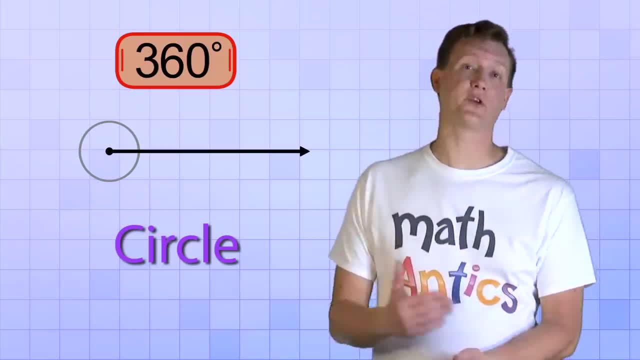 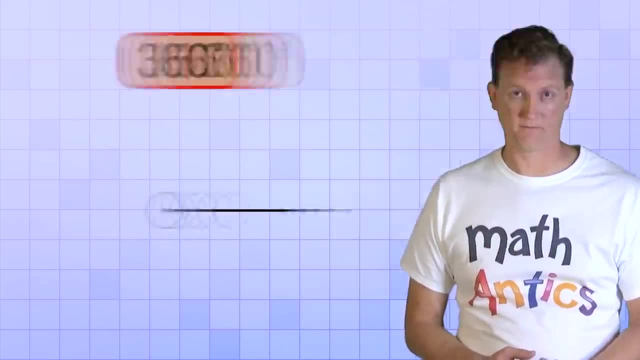 So three hundred and sixty degrees is the angle that represents a full circle. Rotating three hundred and sixty degrees brings you all the way around the circle to the point that you started from. Okay, now that you know what degrees are and you've seen how they relate to the size of an 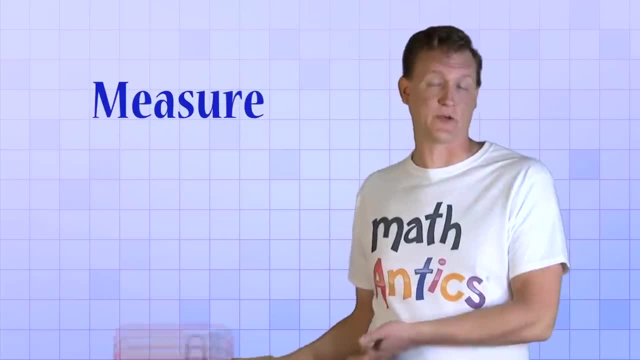 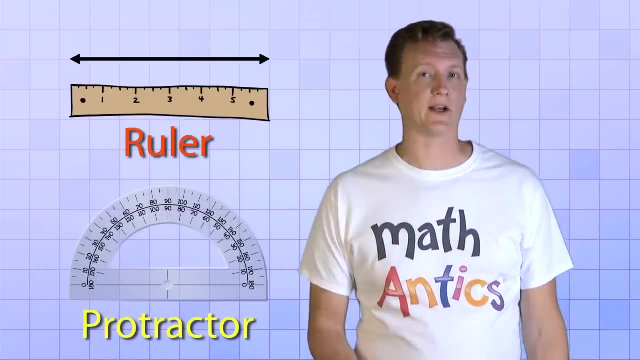 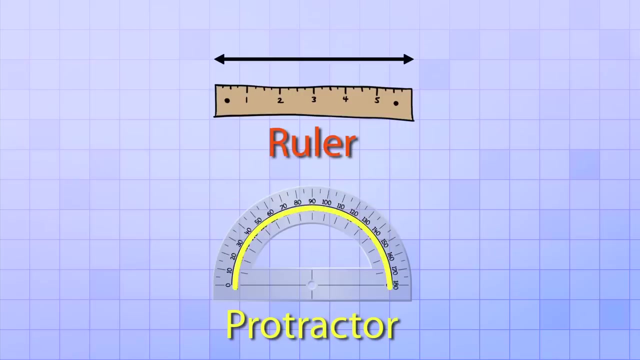 angle. we need to learn how to actually measure an angle without this fancy readout that we have here. A protractor can be used to measure the length of a line. A special tool called a protractor can be used to measure angles. A protractor is similar to a ruler, but it's curved into a half circle, so 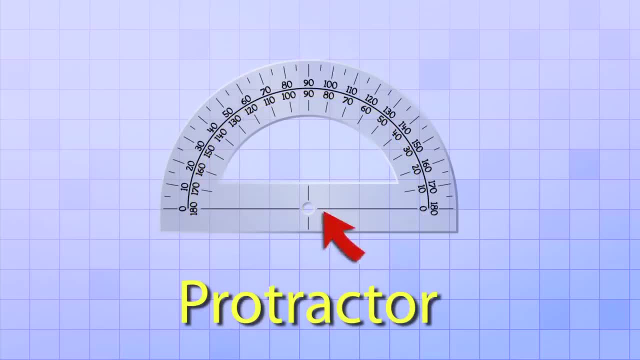 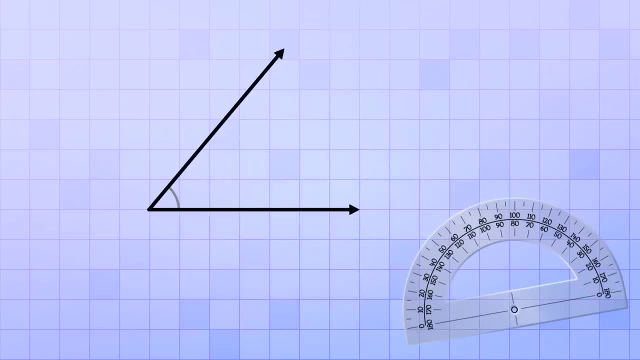 that it can measure rotation around an axis point. A protractor also has a straight edge with a hole or a dot in the middle that represents the axis or center of rotation. So if you're given a mystery angle like this one and you want to measure how many degrees it is, you just put your protractor on. 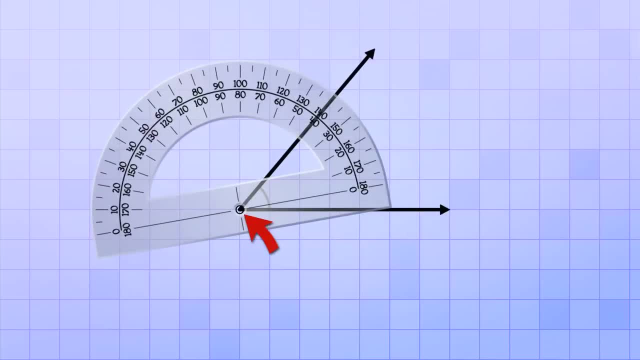 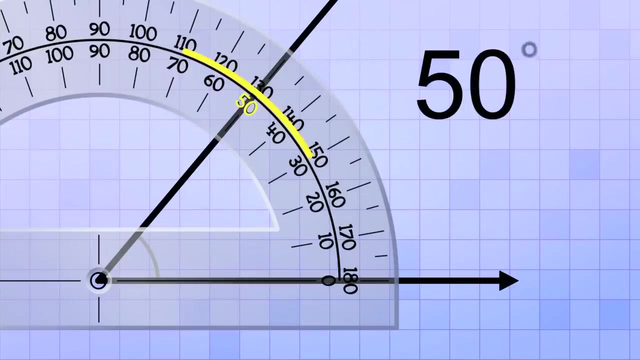 top of it. Then you make sure that one of the rays lines up with the straight line on the protractor And, last of all, you look to see where the other ray crosses the curved part and read off what angle measurement it lines up with. As you can see, this angle here is 50 degrees. 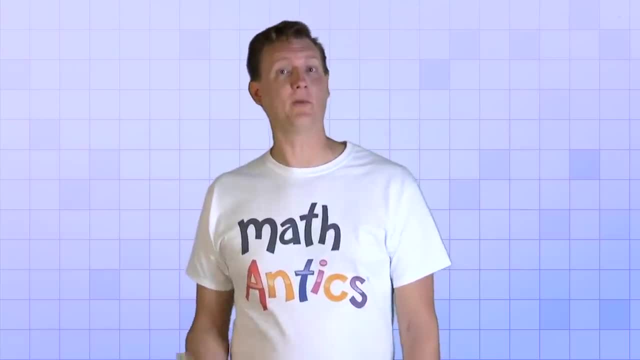 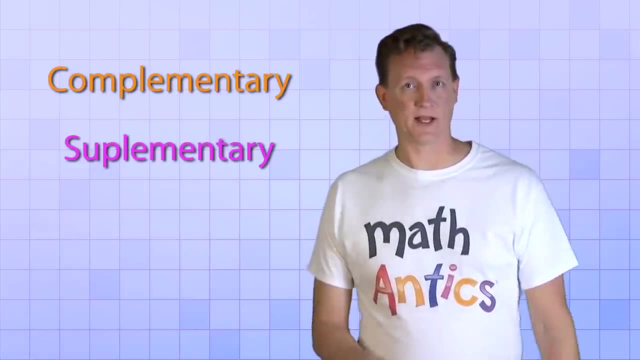 Alright, there's one more thing I want to teach you in this video, because you'll probably see this kind of geometry problem on your homework or tests. Do you remember what complementary and supplementary angles are? from the last video, Complementary angles combine to form a right angle. 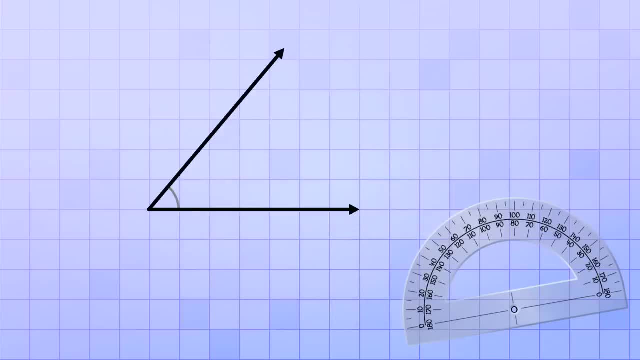 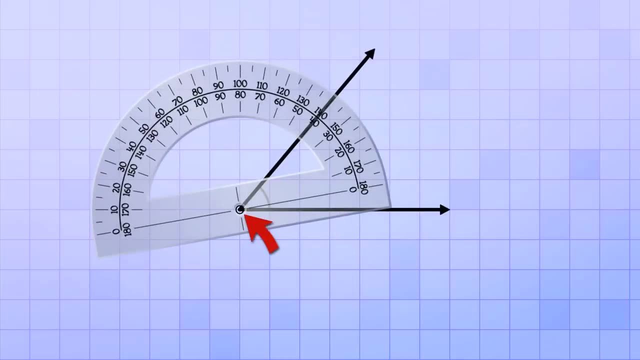 So if you're given a mystery angle like this one and you want to measure how many degrees it is, you just put your protractor on top of it so that the axis point lines up with the intersection of your rays. like this, Then you make sure that one of the rays lines up with the straight line on the protractor. 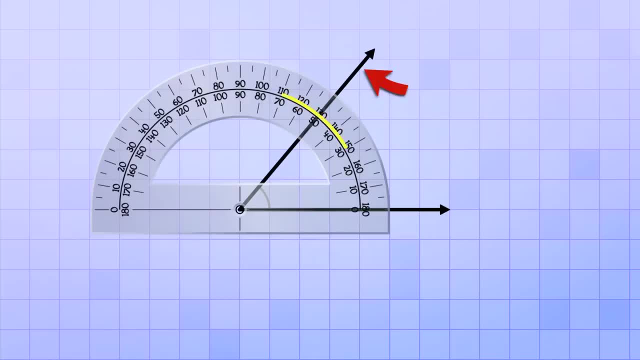 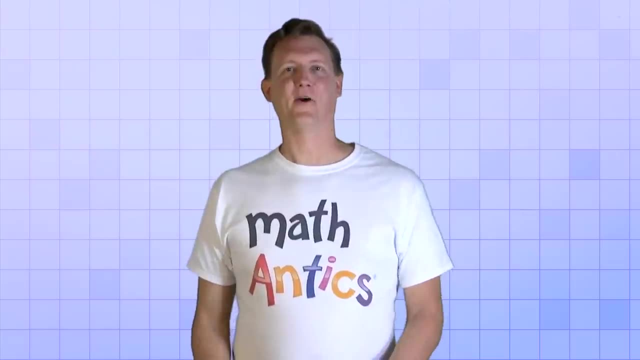 And, last of all, you look to see where the other ray crosses the curved part and read off what angle measurement it lines up with. As you can see, this angle here is 50 degrees. Alright, there's one more thing I want to teach you in this video. 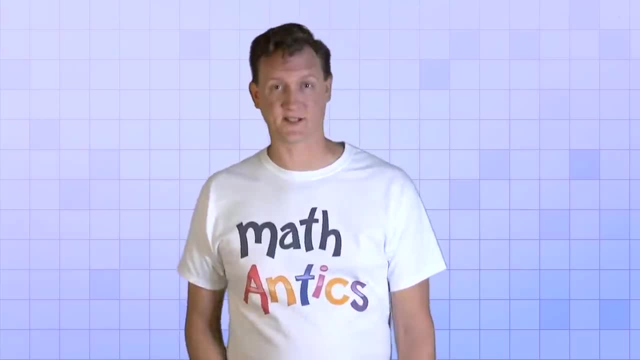 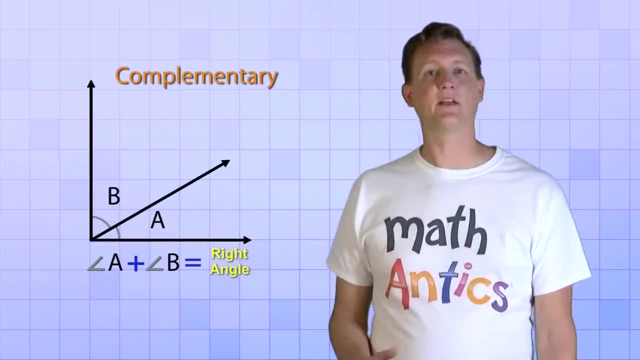 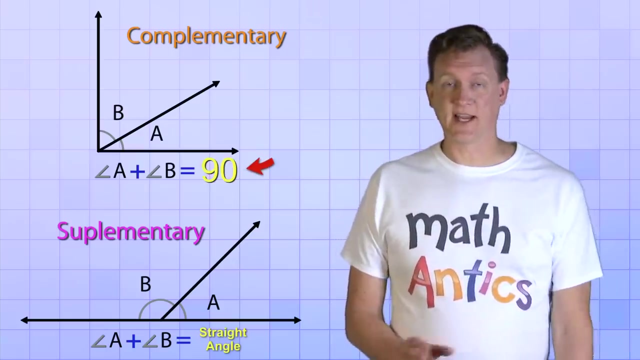 because you'll probably see this kind of geometry problem on your homework or tests. Do you remember what complementary and supplementary angles are? from the last video, Complementary angles combine to form a right angle and supplementary angles combine to form a straight angle. Well, now that we know that a right angle is 90 degrees and a straight angle is 180 degrees, 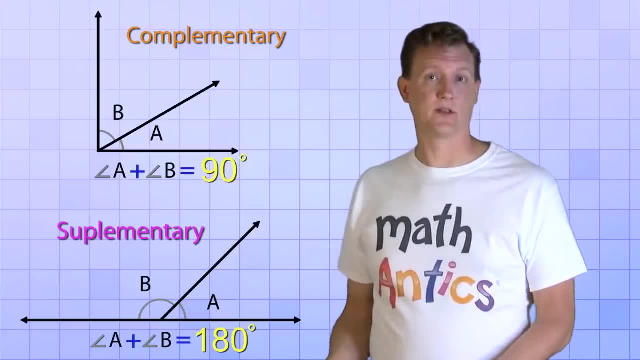 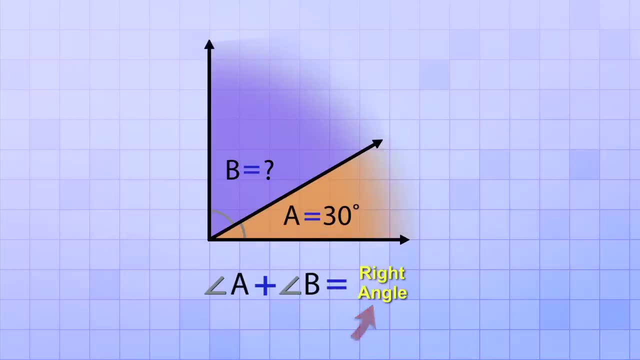 we can use that information to solve problems that have unknown angles, like this one. It shows two angles, angle A and angle B, that combine to form a right angle. The problem tells us that angle A is 30 degrees, and it wants us to figure out what angle B is. 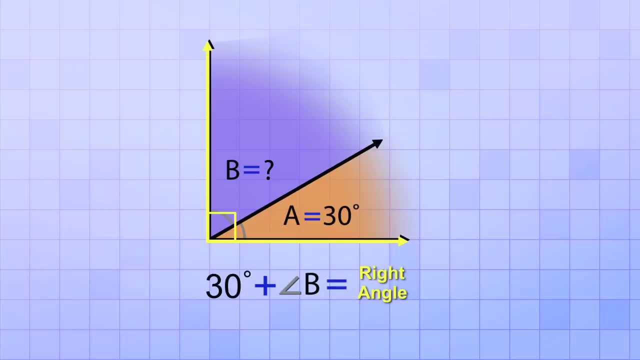 Fortunately, it's easy to figure that out now, because we know that a right angle is 90 degrees, so we know what the total of both angles must be. That means that to find angle B, all we have to do is take the total, which is 90 degrees. 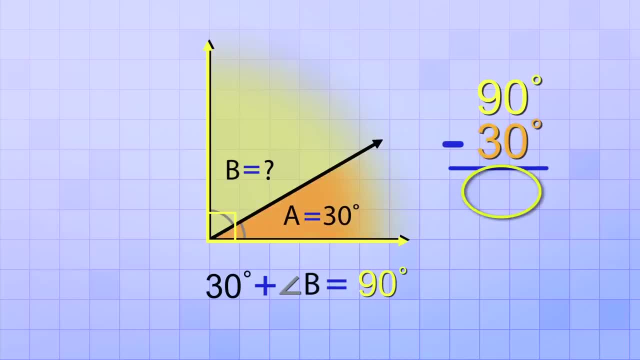 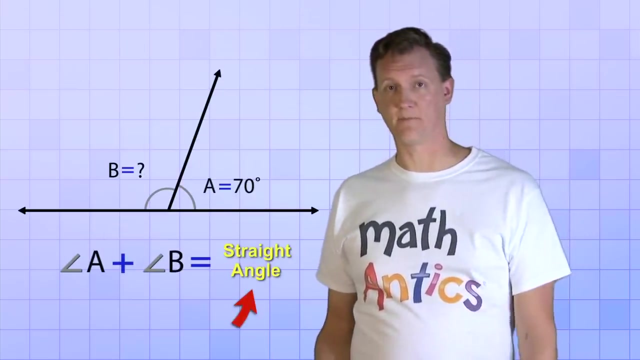 and subtract angle A, which is 30 degrees, and whatever's left over will be the measurement of angle B. So 90 minus 30 equals 60. So angle B is 60 degrees. Now let's try this problem. It uses the same idea, but with a straight angle this time. 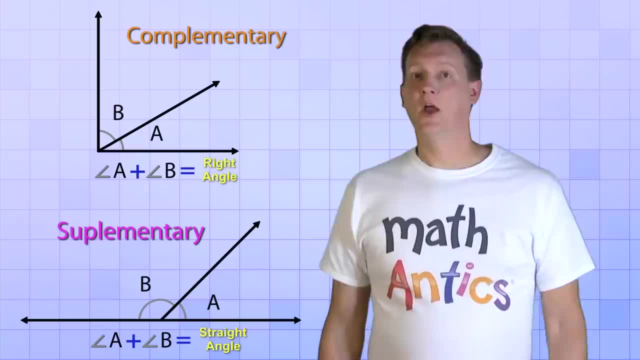 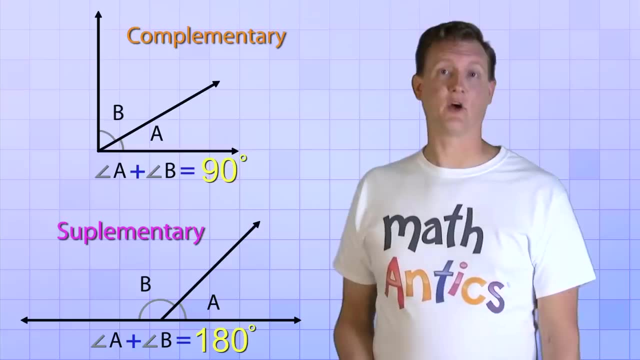 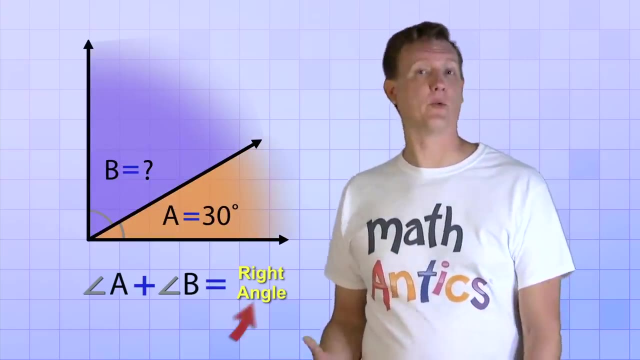 and supplementary angles combine to form a straight angle. Well, now that we know that a right angle is 90 degrees and a straight angle is 180 degrees, we can use that information to solve problems that have unknown angles, like this one. It shows two angles, angle A and angle B, that combine to form a right angle. 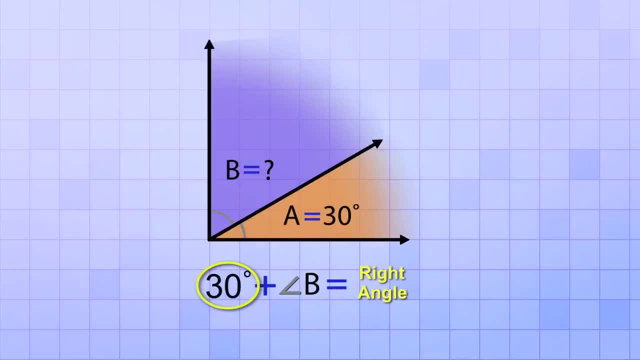 The problem tells us that angle A is 30 degrees and it wants us to figure out what angle B is. Fortunately, it's easy to figure out what angle B is. It's easy to figure that out now because we know that a right angle is 90 degrees. 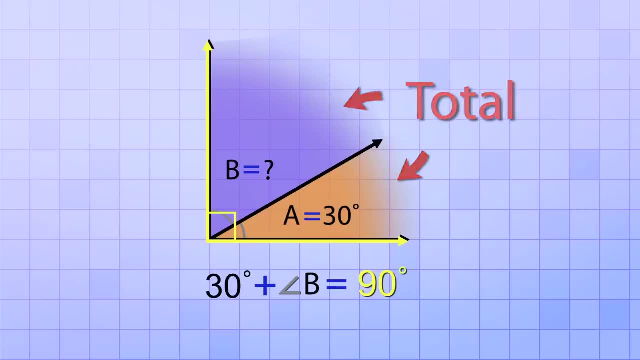 so we know what the total of both angles must be. That means that to find angle B, all we have to do is take the total, which is 90 degrees, and subtract angle A, which is 30 degrees, And whatever's left over will be the measurement of angle B. 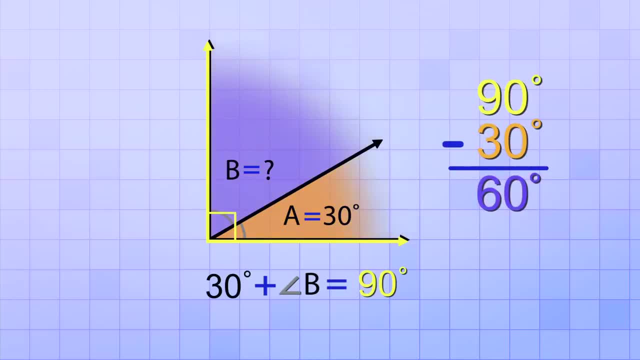 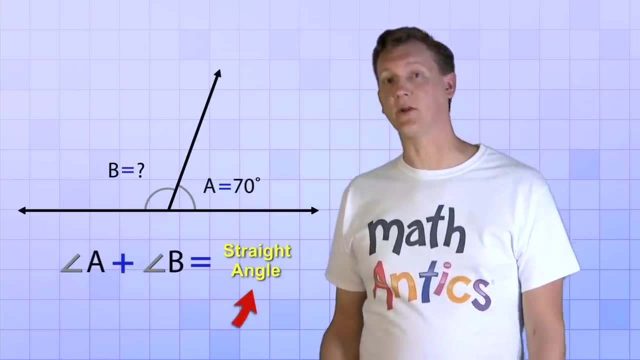 So 90 minus 30 equals 60. So angle B is 60 degrees. Now let's try this problem. It uses the same idea, but with a straight angle. this time The straight angle is divided into two smaller angles again: angle A and angle B. 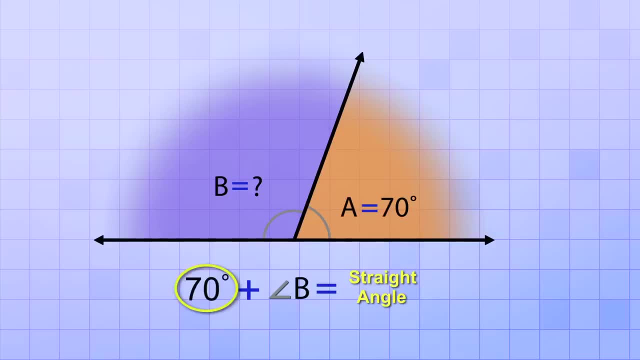 And again the problem tells us that angle A is 70 degrees and it wants us to figure out what angle B is. Well, we know that the total of both angles must be 180 degrees, because we just learned that that's how big a straight angle is. 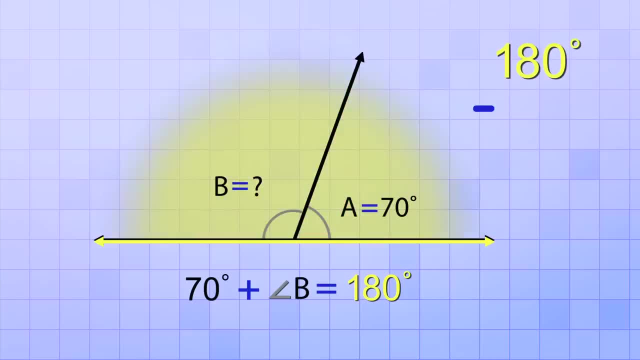 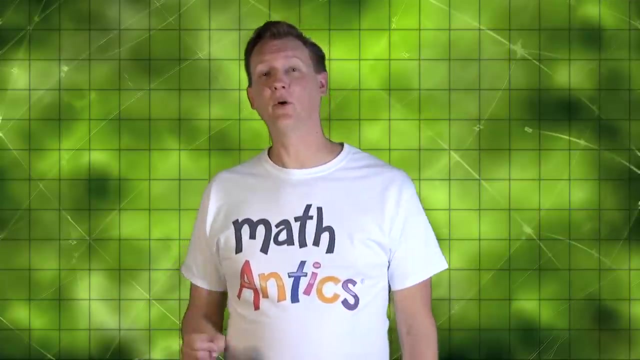 So if we take that total 180 degrees and subtract angle A, which is 70 degrees, whatever's left over after subtracting must be angle B. So 180 minus 70 equals 110.. Pretty cool, huh. And now you can see why it's important to know how degrees work in geometry. 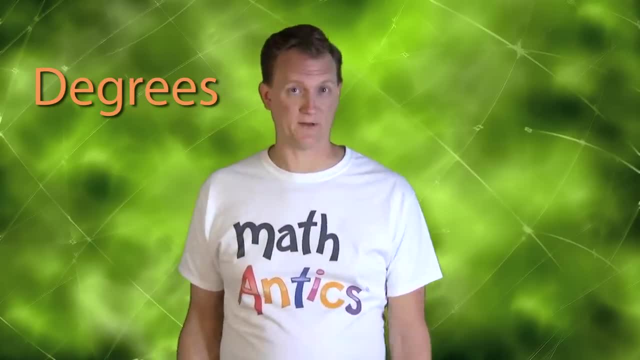 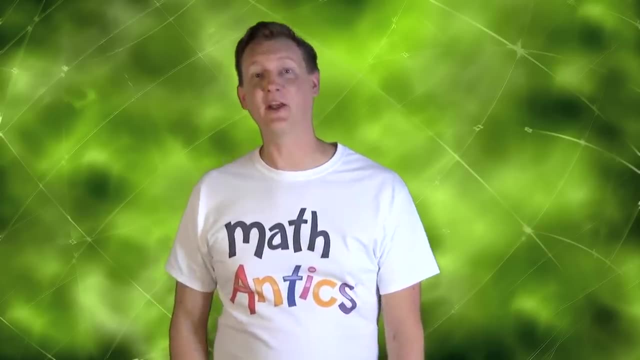 They can tell us how big angles are or how much something is rotated. Well, that's all I've got for you in this video, But, don't worry, there's a lot more geometry where that came from. So I'll get going on my next video and you get going on practicing what you've learned. 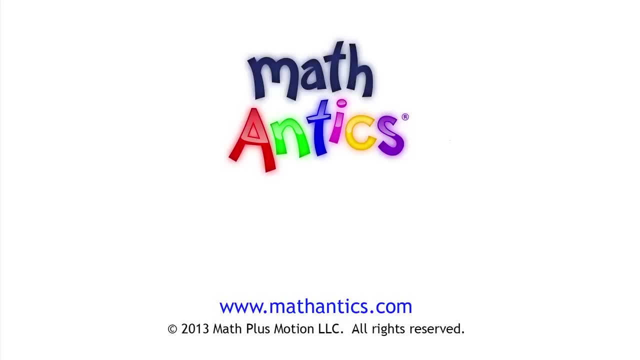 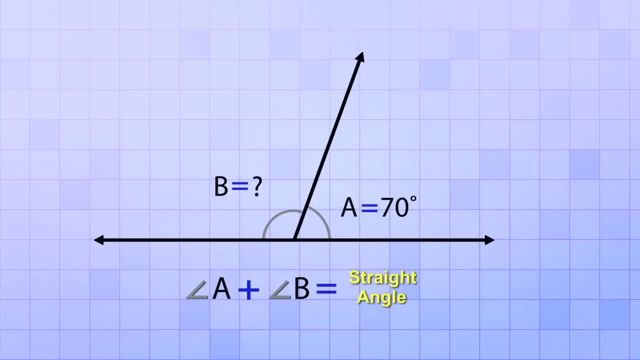 The straight angle is divided into two smaller angles, again angle A and angle B. And again the problem tells us that angle A is 70 degrees and it wants us to figure out what angle B is. Well, we know that the total of both angles must be 180 degrees. 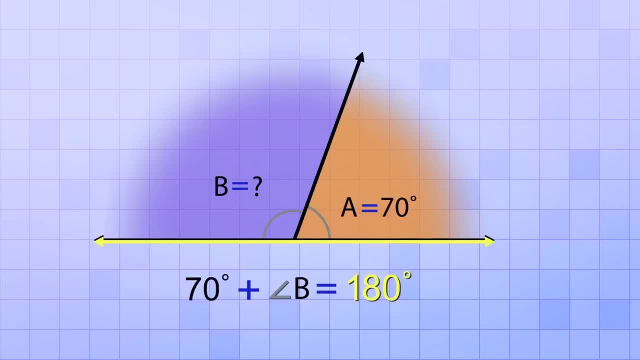 because we just learned that that's how big a straight angle is. So if we take that total 180 degrees and subtract angle A, which is 70 degrees, whatever's left over after subtracting must be angle B. So 180 minus 70 equals 100 degrees.